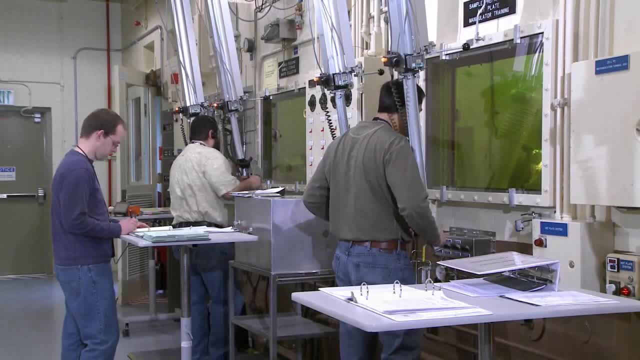 A team of stakeholders, including representatives from maintenance operations, research and development and planning from our major facilities, reviewed these processes. The next is the RAD workers good practice video. This video demonstrates both areas of commonly used cancer and radiological work practices that will no longer be shared with the RWP. 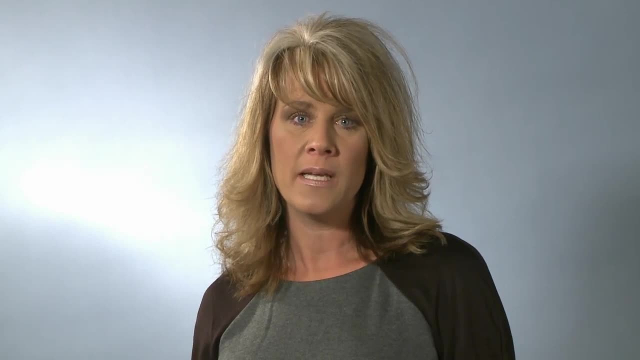 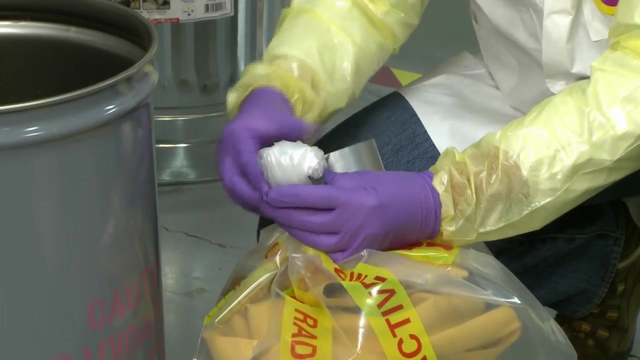 The RAD worker's good practice video is the model video that shows the common use practices that will no longer be covered by the RWP. Much of the information being removed from the RWP is covered in the RAD worker's good practice video. The video demonstrates areas of commonly used practices that will no longer be in the RWP. 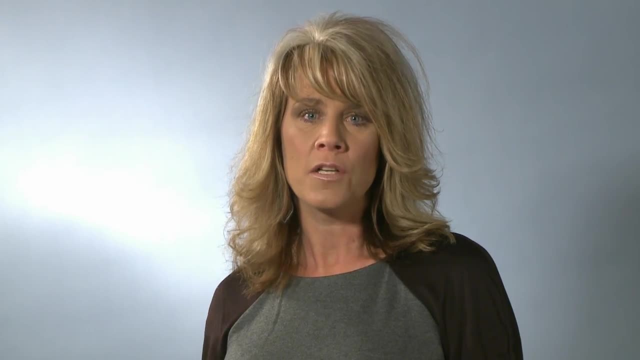 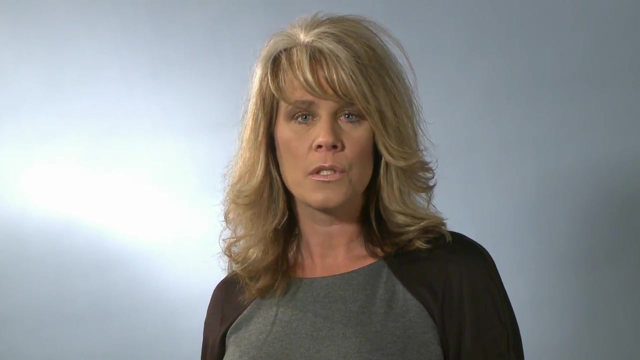 It is expected that RAD workers will be conscientious and use these practices when performing radiological work. The expectation of the radiological control organization is that the Radiological Radio Division of the R&D Unit will provide a neccessary status for RAD workers when performing radiological 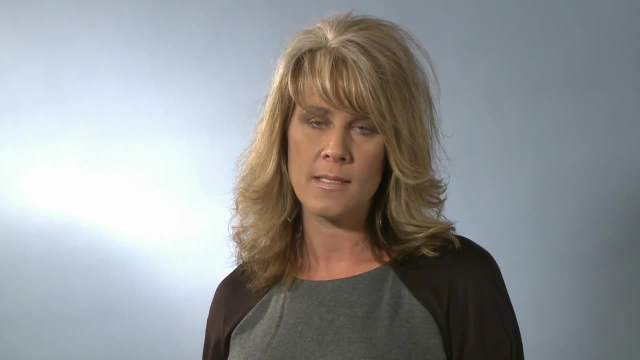 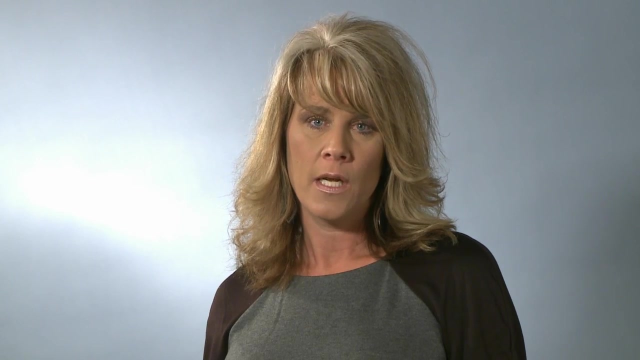 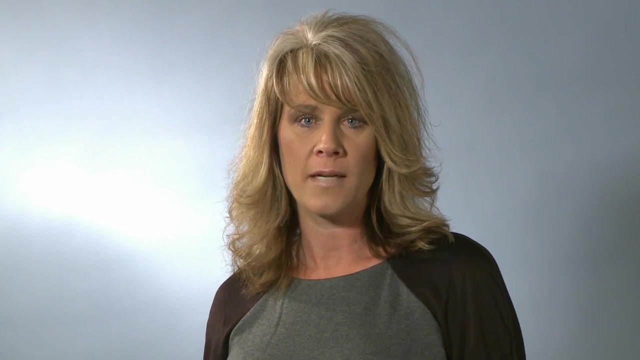 work that we continually strive to improve our processes and ensure the radiological safety of all INL workers. Please take a moment and review the video. You have seen and used many of these practices. We encourage all radiological workers to use these best practices. 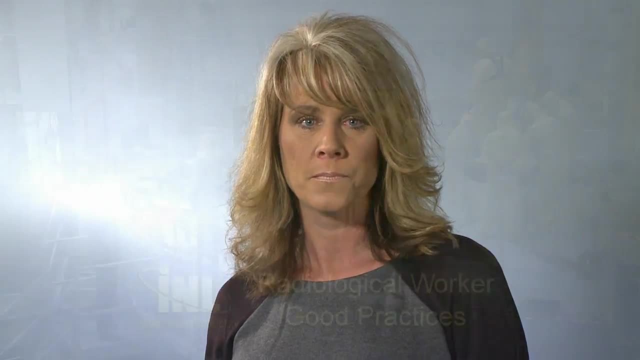 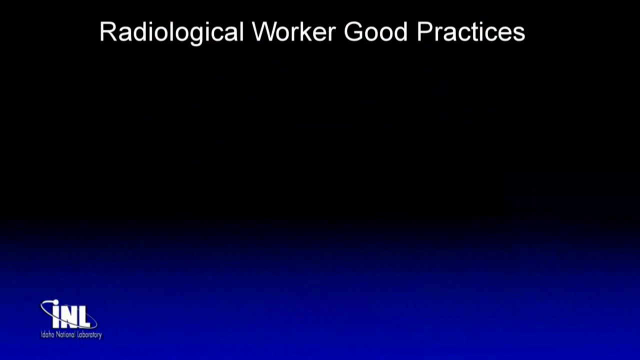 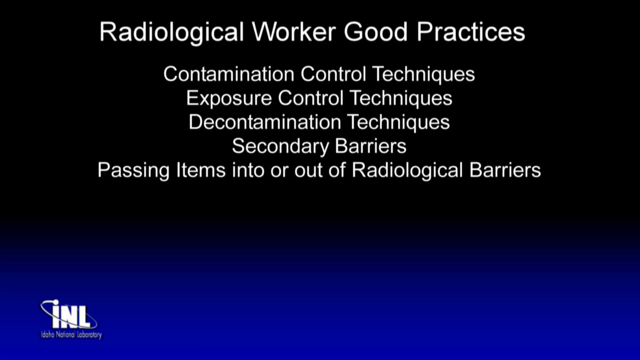 while performing radiological work. Thank you, In this video, radiological worker, good practices have been divided into categories. These categories are: contamination control techniques. exposure control techniques, decontamination techniques. secondary barriers: passing items in to or out of radiological barriers. 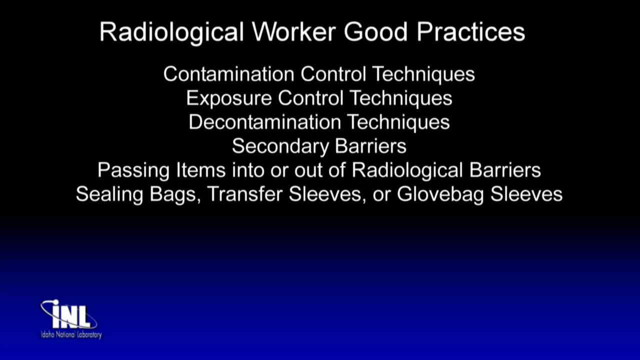 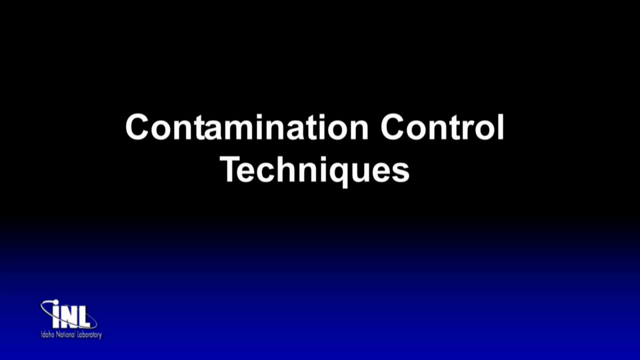 sealing bags, transfer sleeves or glove bag sleeves, glove box work, fume hood work, RAD Worker 101, RWP QPR card or trip tickets and extremity dose tracking card. Contamination control techniques: Techniques commonly used to control contamination. 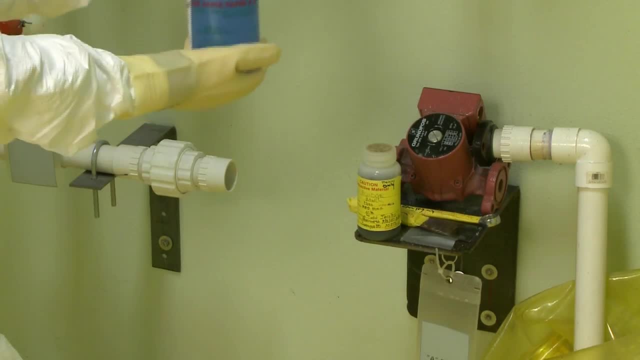 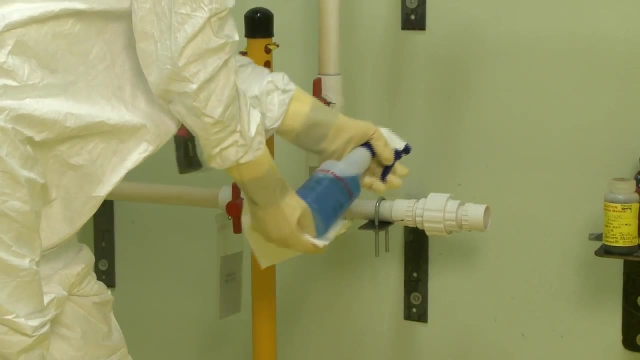 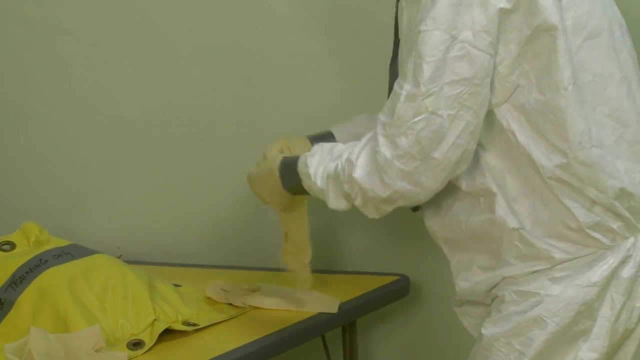 include misting the work area or equipment prior to beginning work. Misting should not be used around electrical equipment or for flighty isotopes. Consult with radiological control personnel before using this technique. Other techniques include changing your gloves frequently during work, as directed by radiological control personnel. 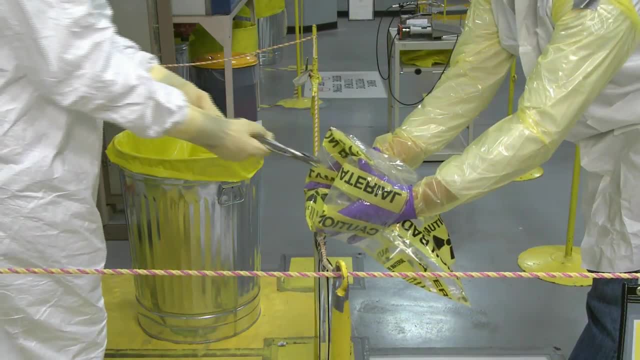 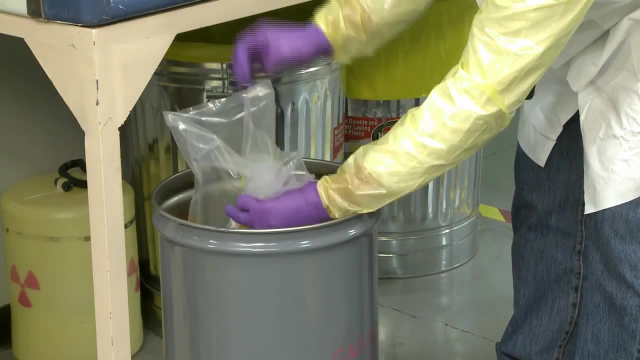 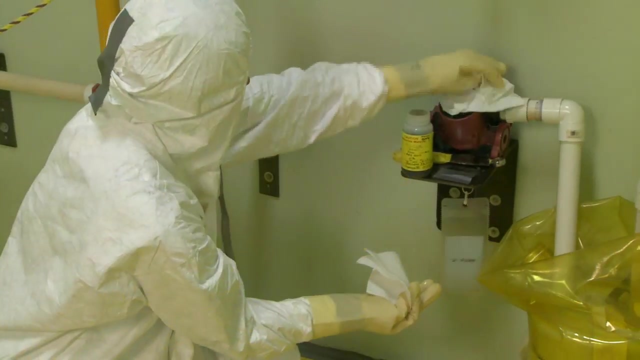 Or, as discussed in the briefing: Bagging contaminated items and waste. Changing out bags and waste cans at three quarters full rather than waiting until they are full or overflowing. Wet mopping floor areas. Wiping down equipment or work area. Taping sharp edges of items before bagging. 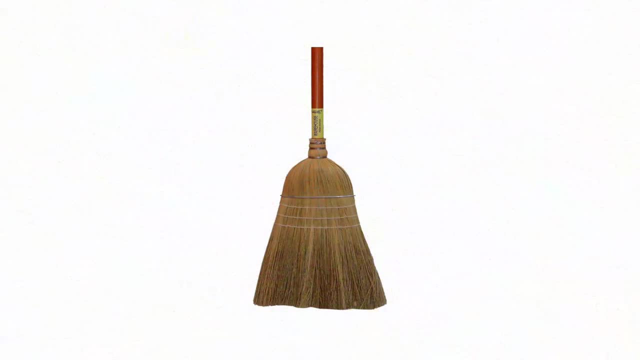 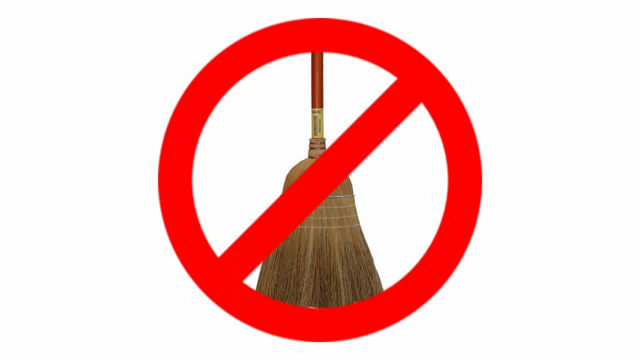 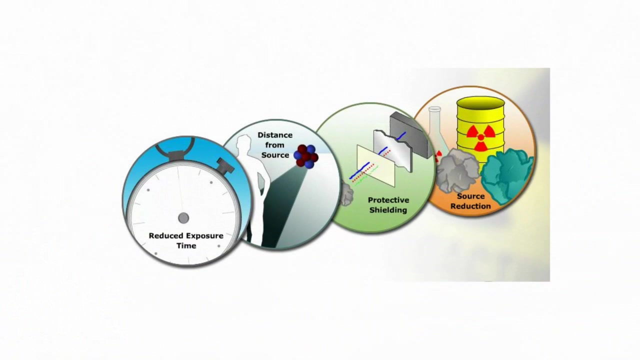 to prevent cutting the bag. Sweeping is not allowed in radiological buffer areas or contamination areas, as this may cause airborne radioactivity Exposure control techniques. Techniques to control exposure are taught in the initial radiological worker training. They include time, distance, shielding and source reduction. 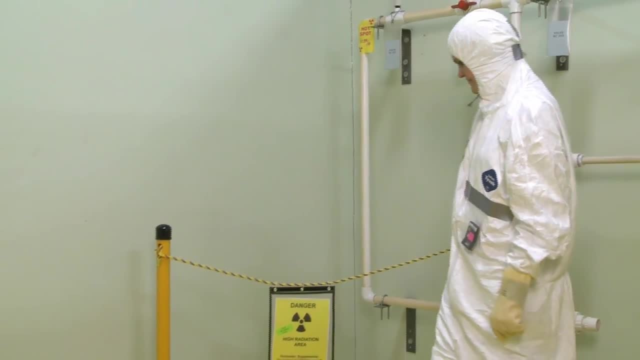 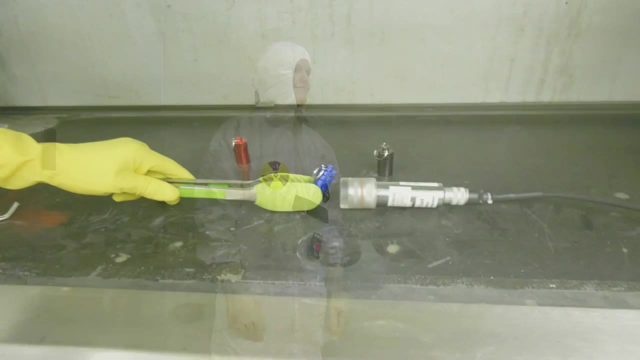 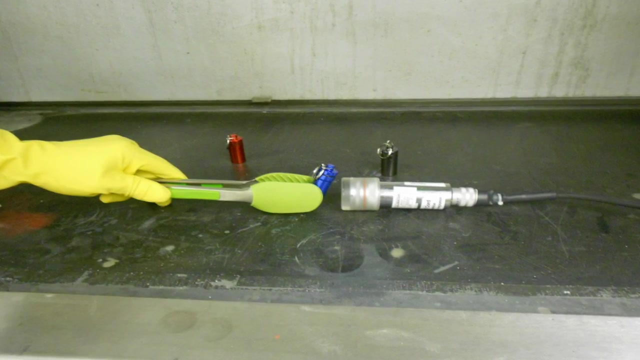 Use low-exposure waiting areas while waiting during radiological work. This will increase your distance and reduce your time near radiation sources. Increase the distance between yourself and the source material using tongs or long-handled tools to reduce your extremity and whole body exposure. 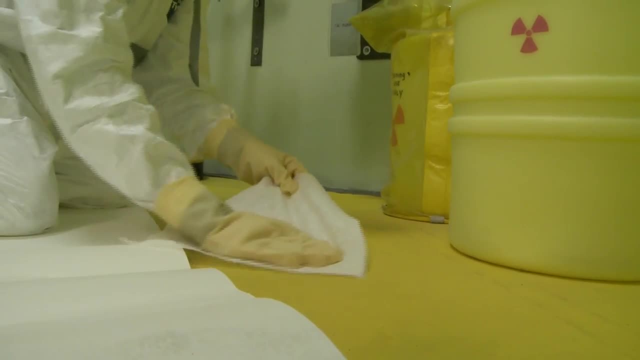 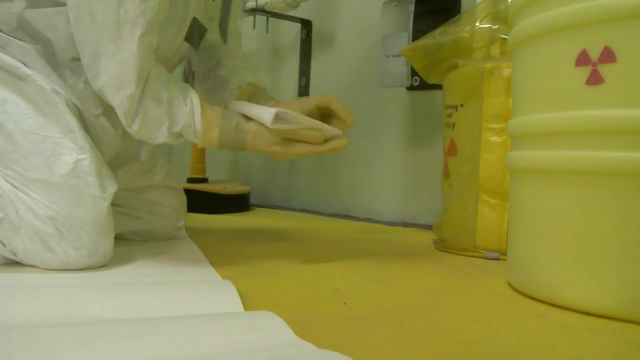 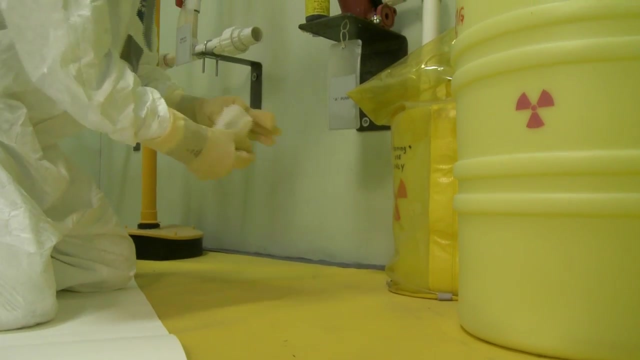 Decontamination techniques. When decontaminating an area or equipment, begin on areas with lower levels of contamination and work toward the areas of higher contamination. Use the wipe and fold technique, concentrating on contamination removal rather than just smearing it around around. 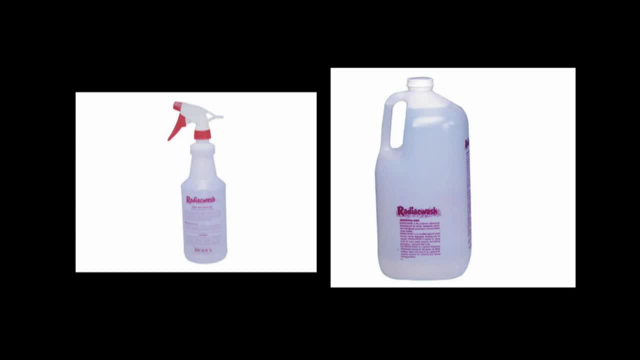 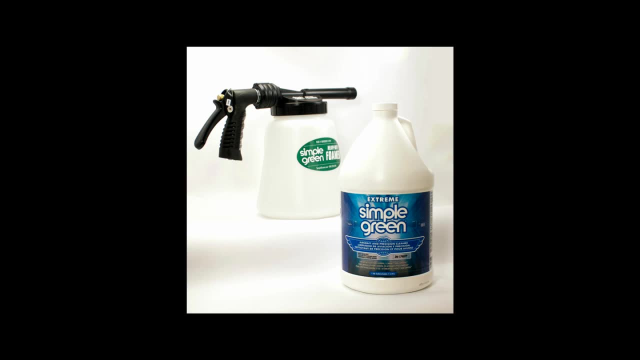 You may also consider the use of commercially available decontamination solutions such as Radiac Wash If the contamination is trapped in greaser oil. a solvent-based cleaner such as Extreme Simple Green Aircraft and Precision Cleaner is helpful to dissolve and break down the greaser oil. 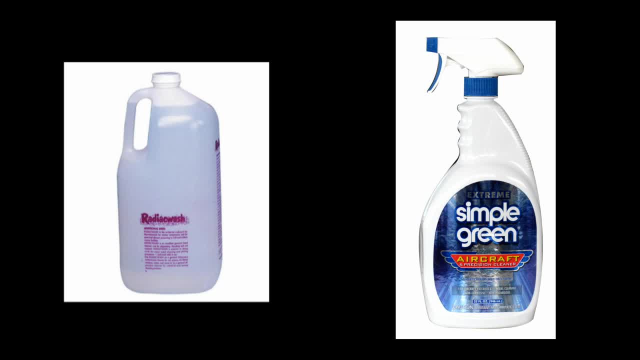 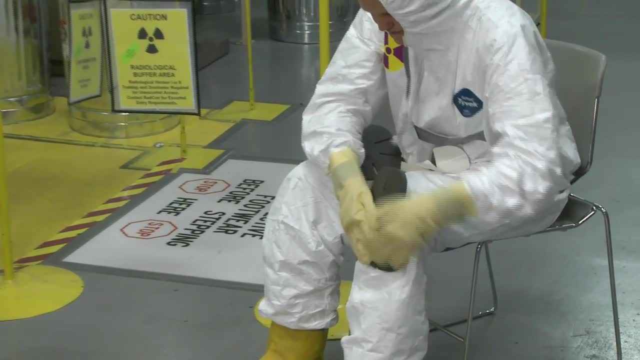 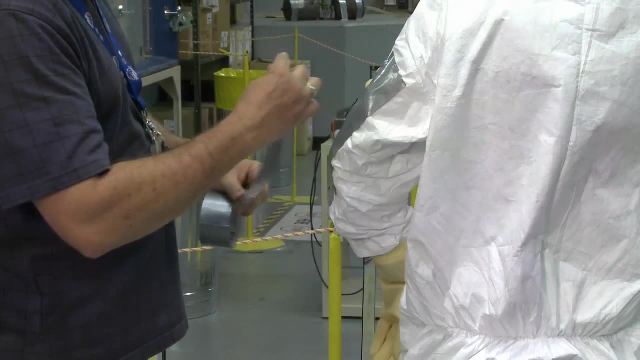 Ensure you obtain facility management and industrial hygiene approval to use any decontamination agent or solution. Secondary barriers: Examples of secondary barriers used in conjunction with personal protective equipment would include the use of adhesive knee pads. taping over the pressure points, such as knees and elbows, with duct tape. 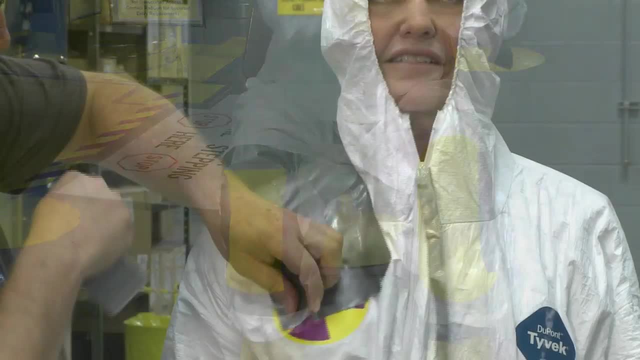 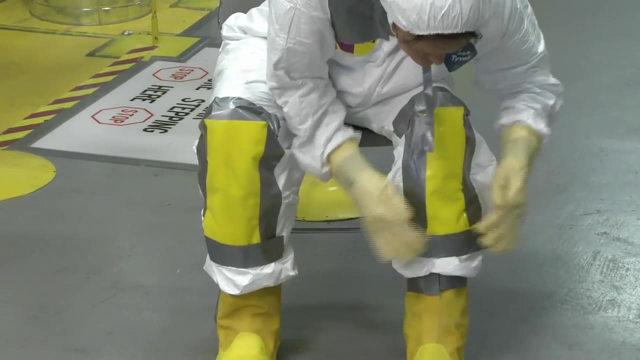 taping plastic shoe covers over at the knees. taping over the shoulder area to rest long-reach tools on the shoulder. These barriers need to be moisture impervious to prevent wicking of contamination. Other examples of secondary barriers would include using poly sheeting. 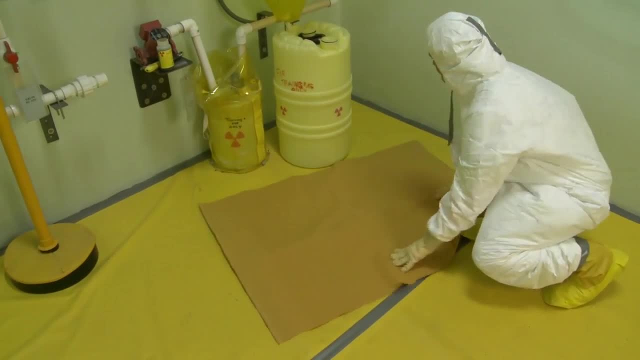 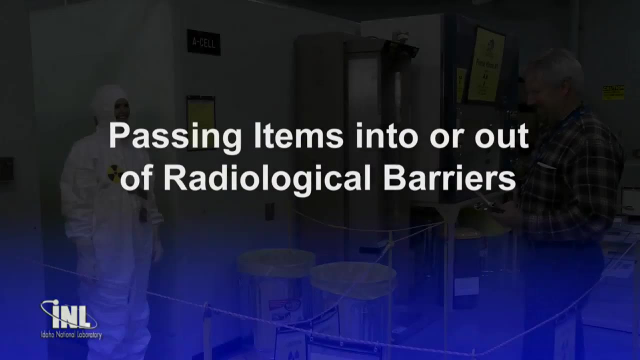 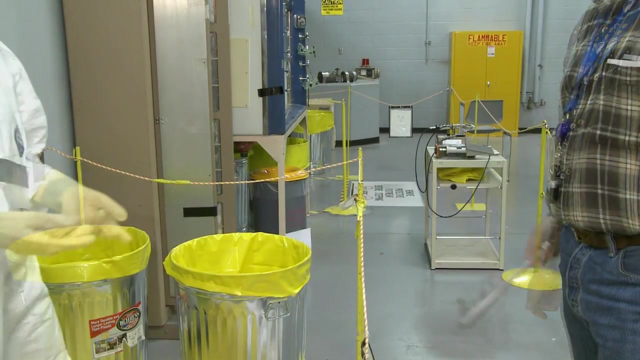 blotter paper or tacky cloth to cover equipment or the floor of the work area. Passing items into or out of radiological barriers. To pass items into a radiological buffer area or contamination area, hand the item across the barrier without the sender or receiver allowing their hands. 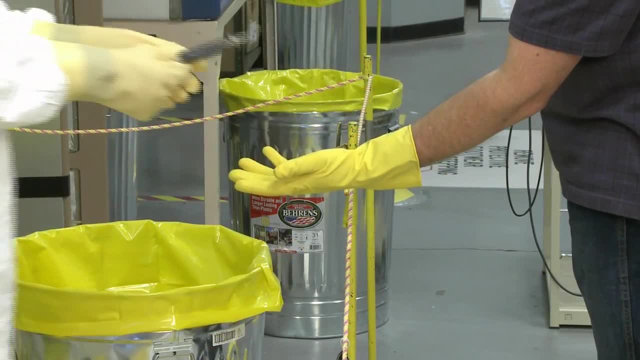 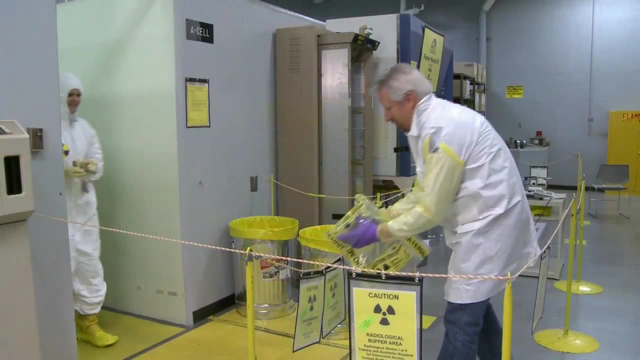 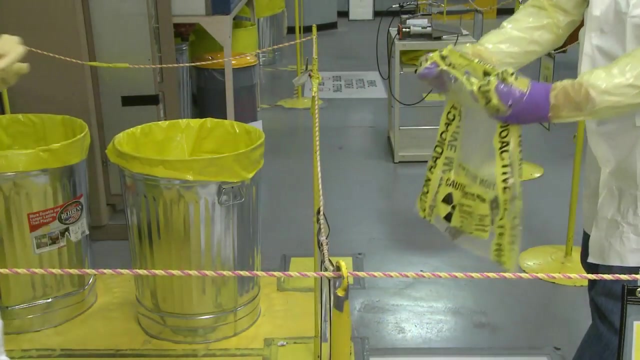 to break the vertical plane of the barrier To pass items out of the radiological barriers. the receiver receives the item into a gloved hand or into a plastic bag. The sender should not break the vertical plane of the barrier with either the item being passed out or with their hands. 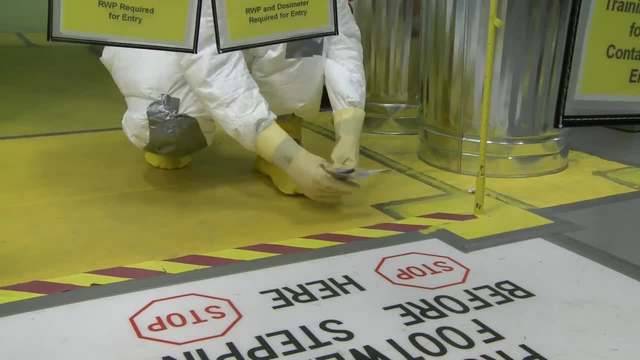 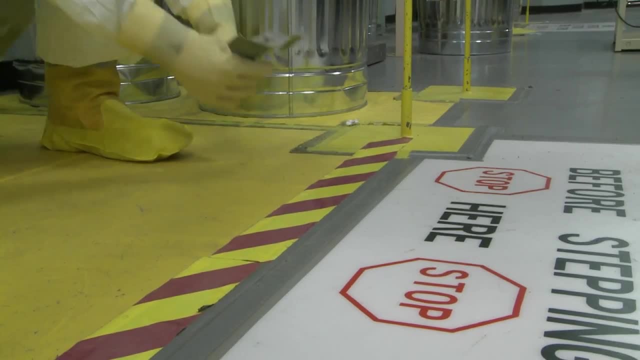 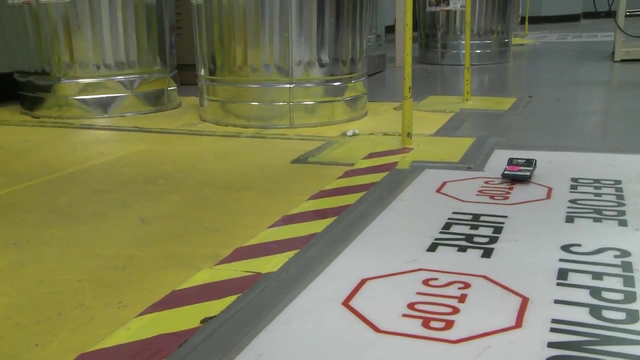 To pass out an ED without HPT or RCT assistance without breaking the barrier plane. with your hand, squeeze the ED out of the bag and onto the ED tray at the barrier if present, or onto the step-off pad if no tray is present. 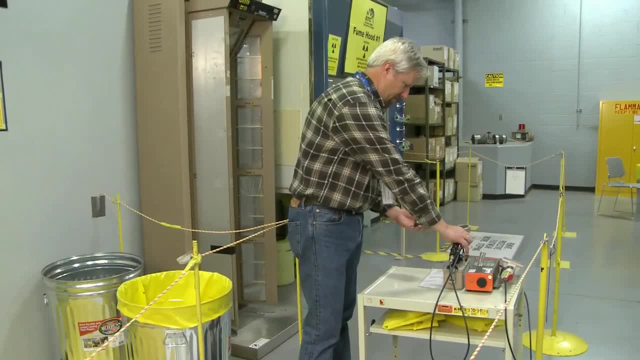 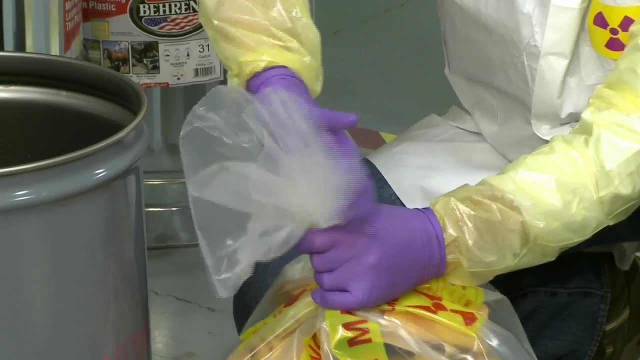 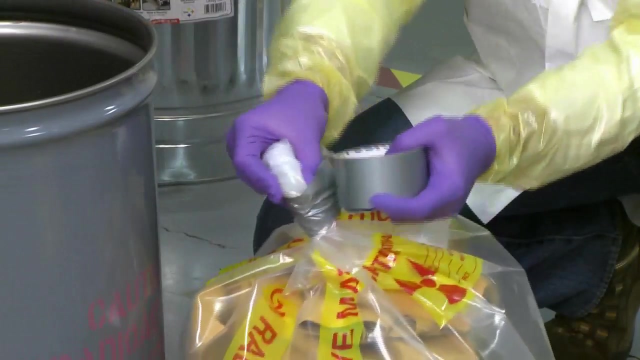 The ED must be surveyed prior to removal from the radiological buffer area. Sealing bags, transfer sleeves or glove bag sleeves. A J-seal is performed by twisting the open end of the bag or sleeve into a tight twist, taping around the twist, then folding the end. 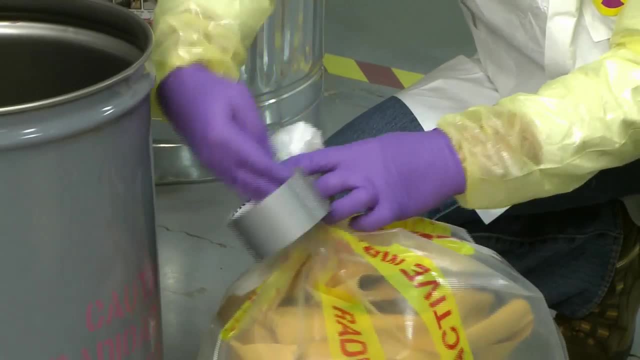 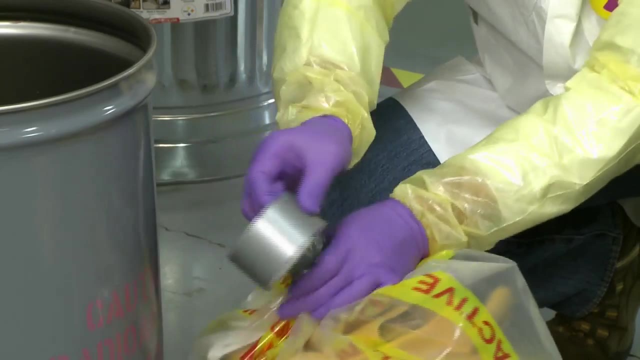 of the bag or sleeve forming a J and then taping the end, sealing that end, closed. Do not squish the air out of the bag as this may release contamination. A twist and tape seal is performed by twisting the sleeve into a tight twist. 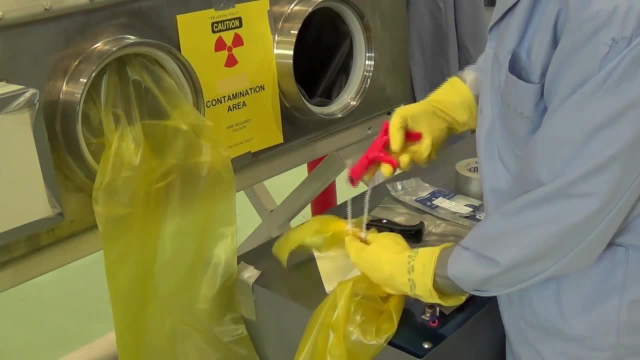 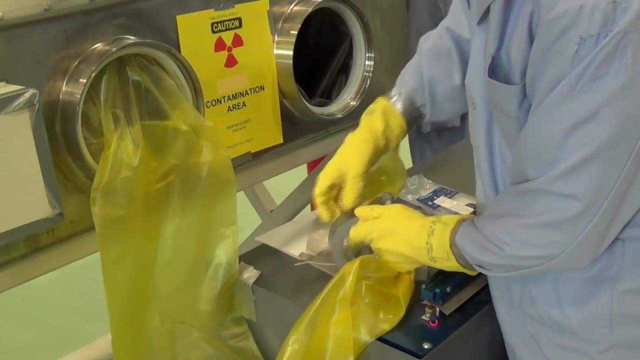 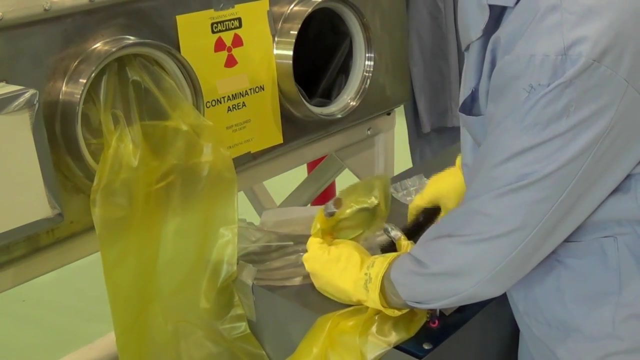 tightening a cable tie on each side of the twisted sleeve to be cut, then taping around the twisted sleeve and cable ties. Next prepare duct tape crosses to cover the ends of the sleeve, then cut through the twisted sleeve and duct tape and apply these taped crosses over the cut ends. 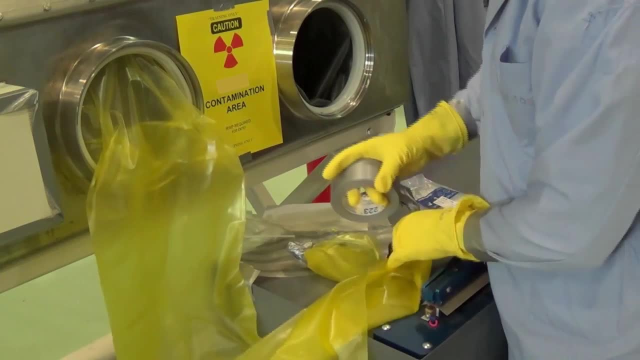 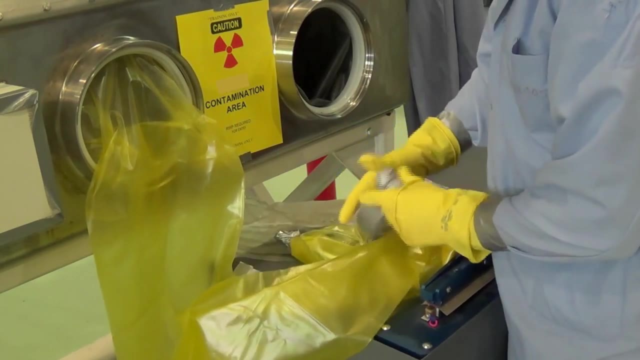 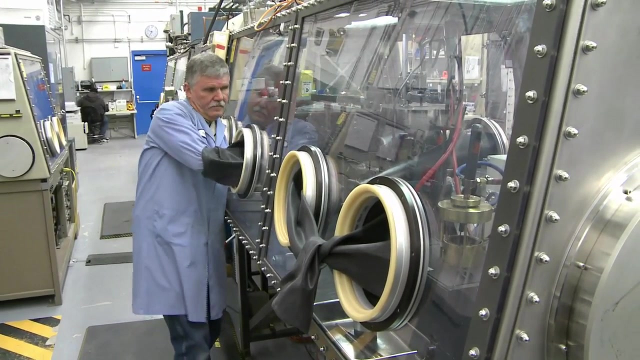 The last step is to tape around the ends of the taped crosses and have an HPT or RCT survey. the cutter and sleeving ends for contamination Glove box work. In preparing to work in a radiological glove box, look for sharp objects and pinch points. 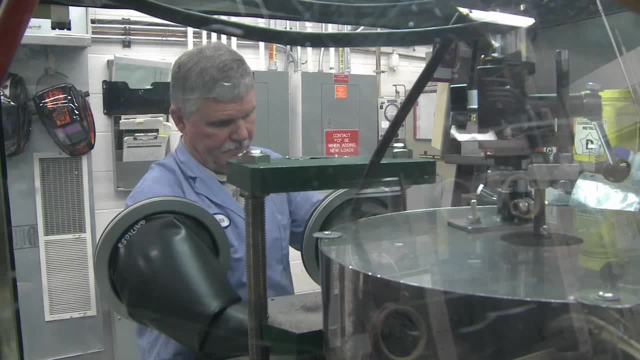 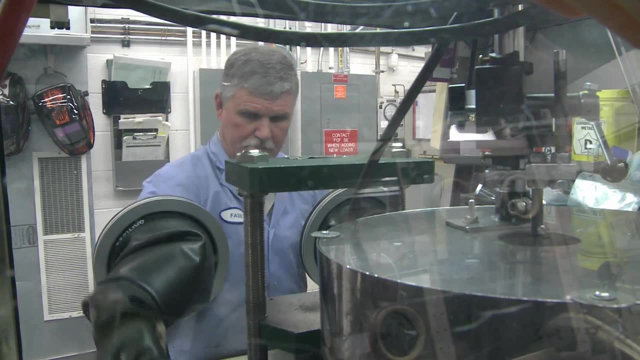 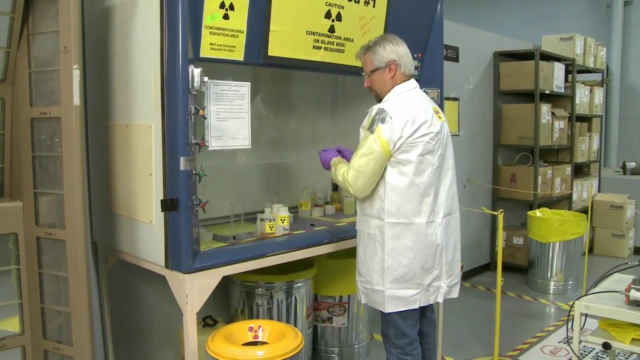 Ensure that unnecessary materials and equipment is out of the way. Ensure flammable materials are not present. Ensure that all required material, equipment and tools are staged for the work. Fume hood work. Ensure the waste can is positioned in a close proximity to the hood face.